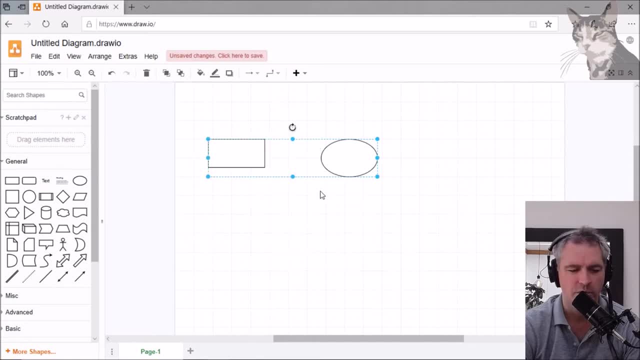 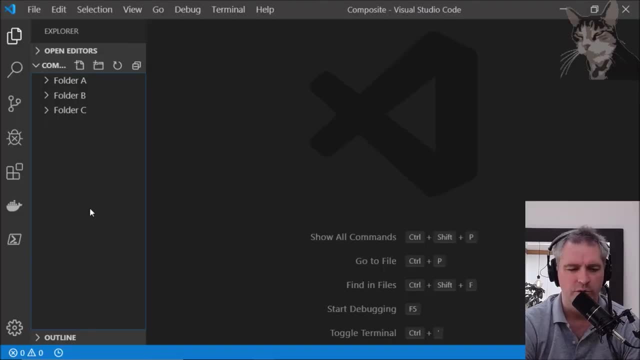 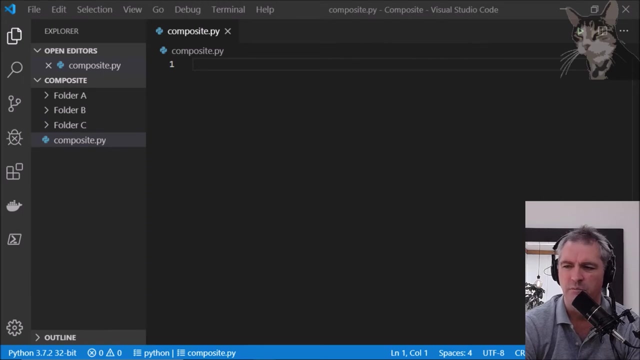 So we can group those two entities Group. And now they are a composite So I can move them both around. Let's start coding. First thing I'm going to do is create a new file called compositepy. In that file I'm going to add the abstract metaclasses. 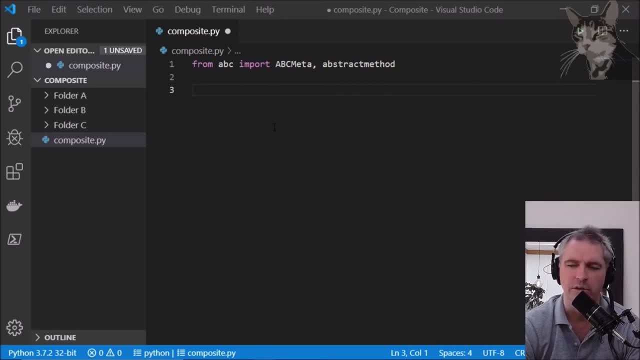 I'm going to create an example which most closely resembles the drawing application I just showed. So I'm going to have an interface called iGraphic- And this is the entity, The entity interface, with one method called print, And that's an abstract static. I'm going to create one entity called an ellipse, Which implements: 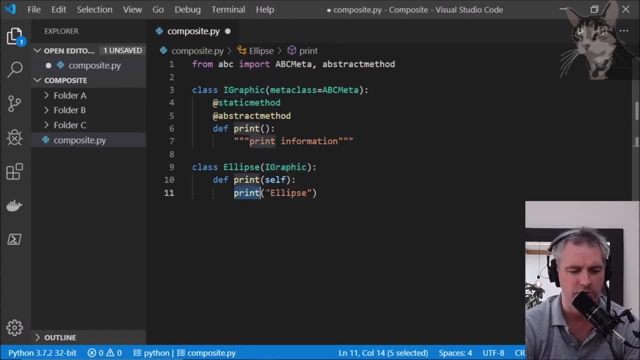 the iGraphic interface And it prints the word ellipse. I'll create another Entity called a circle, Which also implements the iGraphic interface and prints circle. Okay, that's good. Now let's create a composite which also implements the iGraphic interface. 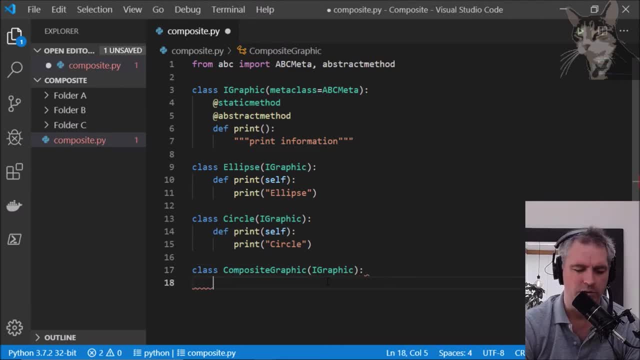 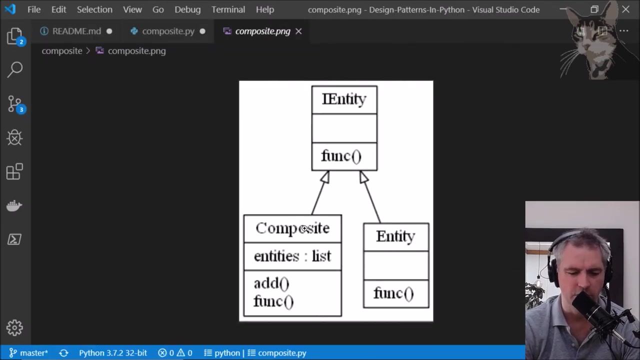 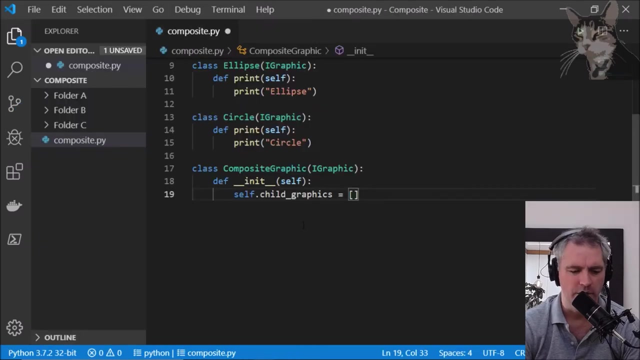 Okay so class composite: graphic implements iGraphic. Has an int. Has an init. Graphics equals a list. So this is going back to our image. We're creating our composite, which has an aggregate or a list or a collection of entities. Add a method to add entities. So 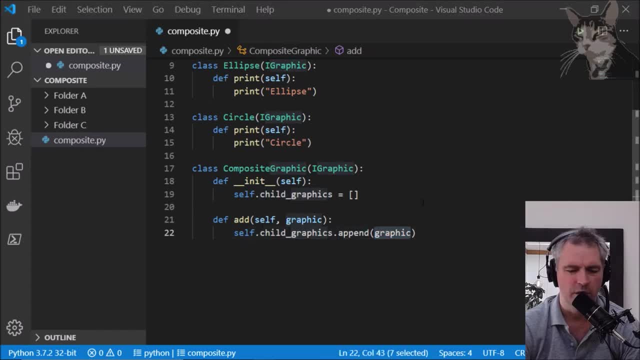 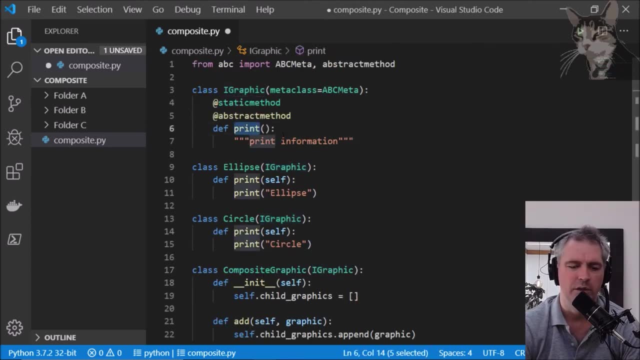 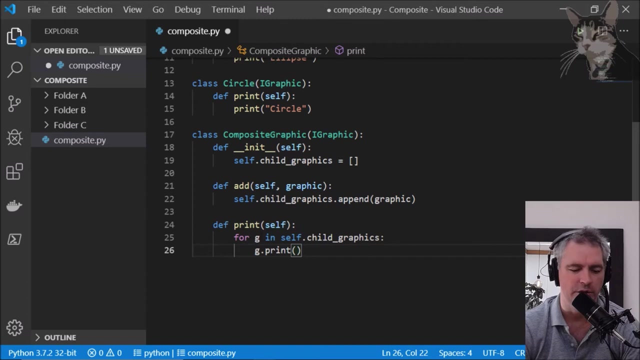 childgraphicsappend a graphic, And because it implements the iGraphic interface, we must add the print method. So let's do that now: Print self for each of the child entities in the child graphics. We'll run its print method. So let's create a client that uses all that. 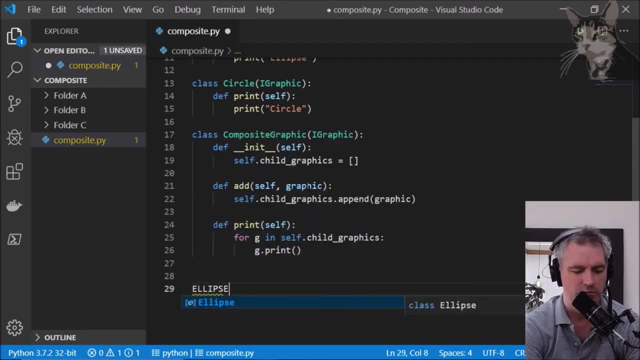 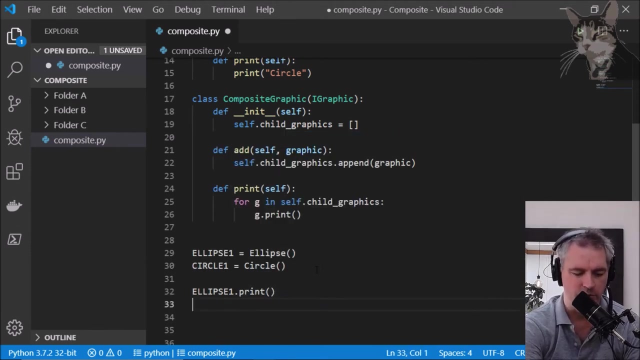 So I'm going to create an ellipse- Ellipse one equals an ellipse. Let's create a circle. A circle one Equals a circle, And for ellipse we can, we can run the print method, And for circle we can also run the print method. So let's try that out.